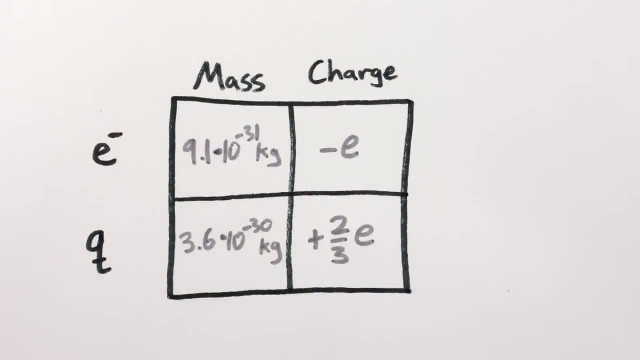 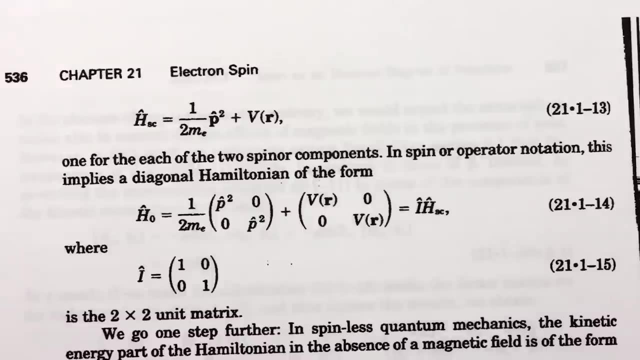 have fundamental properties called mass and electrical charge. most particles also have another intrinsic property called tiny magnet. Just kidding, It's called intrinsic magnetic moment, But really that's just technical mumbo jumbo saying that particles with electric charge also happen to be tiny magnets. If you want to know why they're tiny magnets, well, you may as well ask: why are particles charged in the first place? Or why do objects with mass and energy attract each other gravitationally? No one knows. We just know that's the way the universe works. 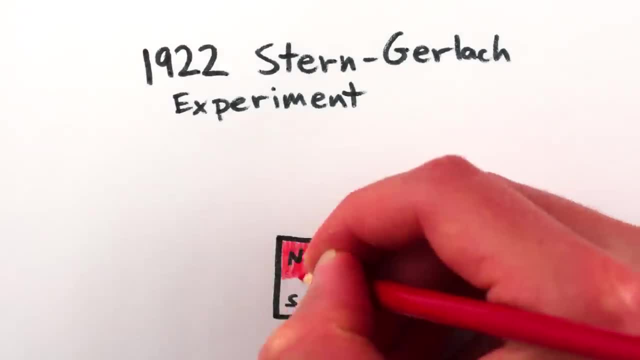 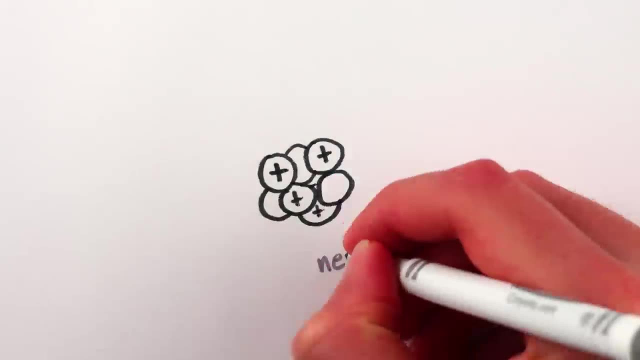 Exactly, And since the 1920s we've known that each individual electron or proton is basically a tiny magnet which brings us to the level of atoms. An atom is a bunch of positively charged protons with a bunch of negatively charged electrons whizzing around them. 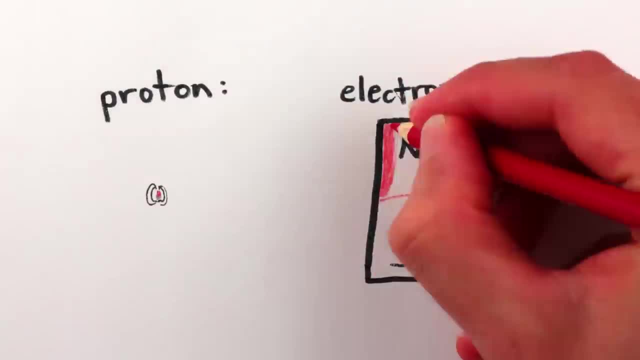 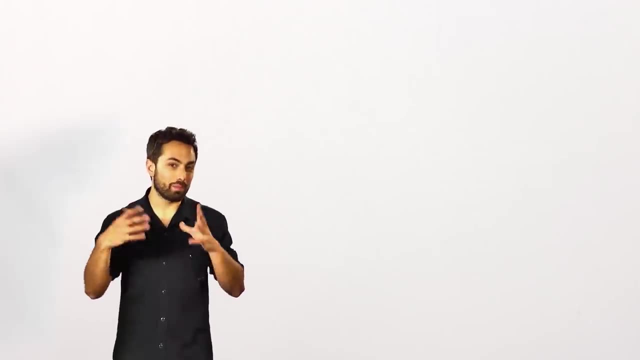 The proton tiny magnets are about a thousand times weaker than the electron ones, so the nucleus of the atom has almost no effect on the magnetism of the atom as a whole. And you might think that since many, though not all, of the electrons are also moving, that like the current in a wire. 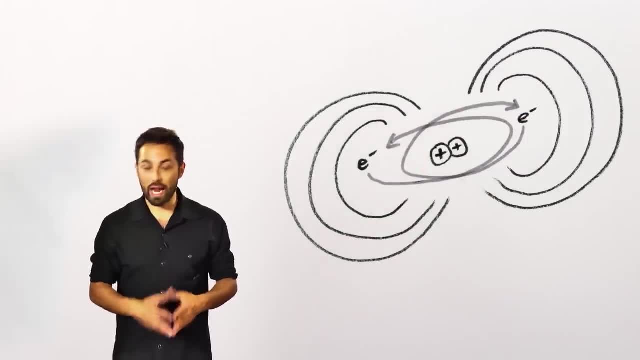 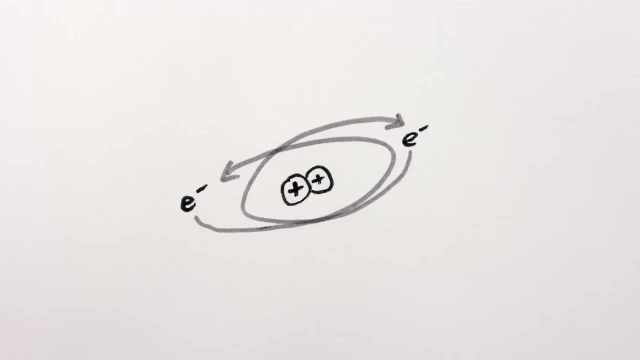 they should generate magnetic fields due to that motion, And indeed they do. These are called orbital magnetic fields. Except, these don't usually contribute to the magnetic field of an atom. Here's why Electrons in atoms are accurately and complicatedly described by quantum mechanics. 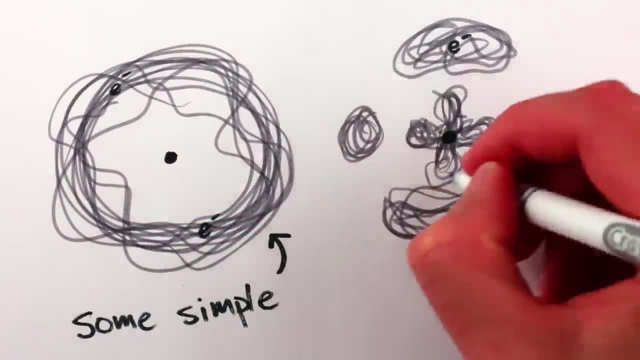 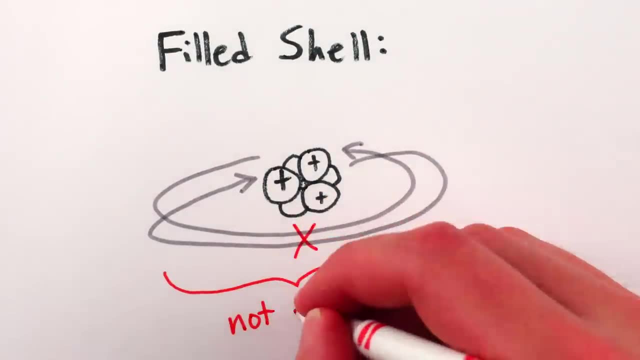 but the gist of the story is that electrons congregate in shells around the nucleus. The electrons in any filled shell zoom equally in all directions, so the currents they generate cancel out And generate no magnetic field. These electrons also come in pairs whose tiny magnets point in opposite directions and also cancel. 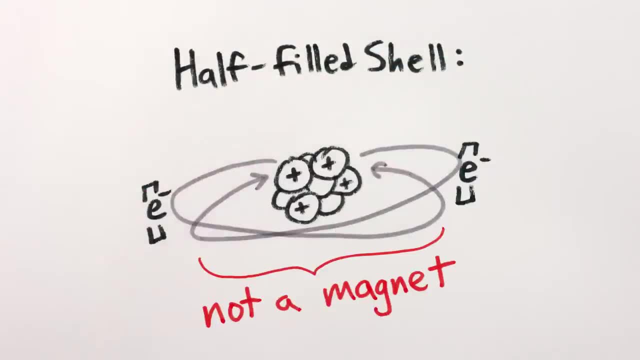 However, in a half-filled shell, all of the electrons are unpaired and their tiny magnets point in the same direction and add up, Meaning that it's the intrinsic magnetism of the electrons in the outer shell that gives an atom the majority of its magnetic field. 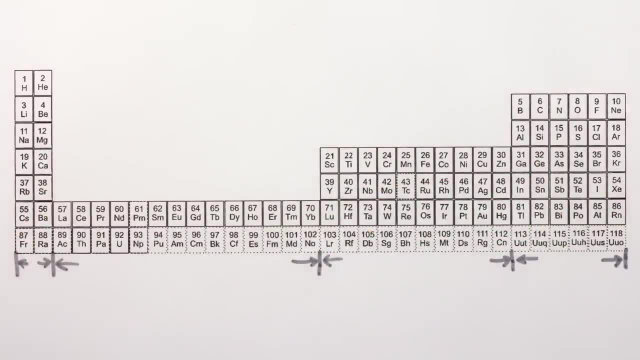 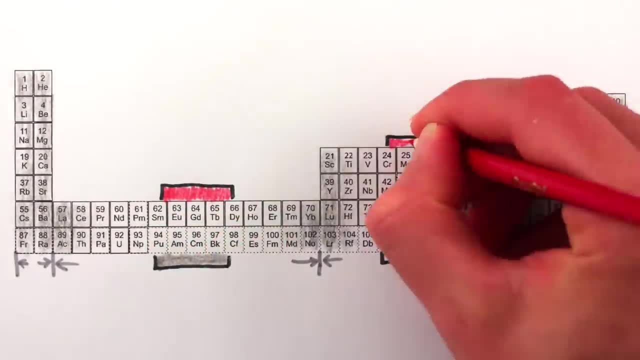 So atoms near the side of any of the major blocks of the periodic table which have full or nearly full outer electron shells aren't magnetic. And atoms in the middle of the block have half-full outer electron shells and are magnetic, For example nickel, cobalt, iron, manganese, chromium, etc. 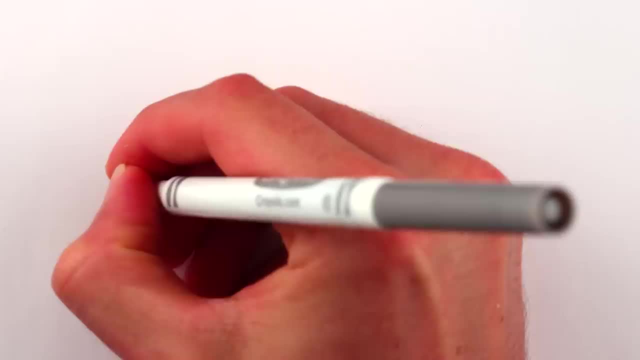 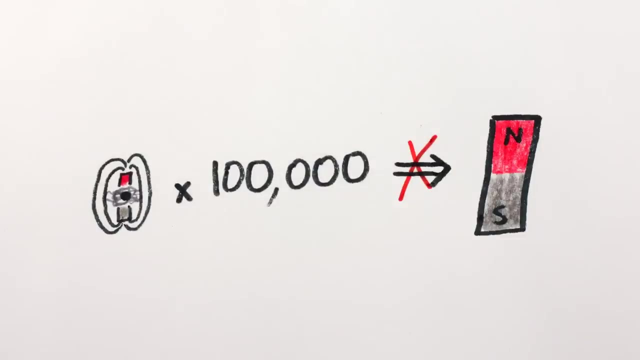 Wait, but chromium isn't magnetic. Ah, but just because an atom is magnetic doesn't mean that a material made up of lots of that atom will be magnetic, Which brings us to the level of crystals, When a bunch of magnetic atoms get together to make a solid. 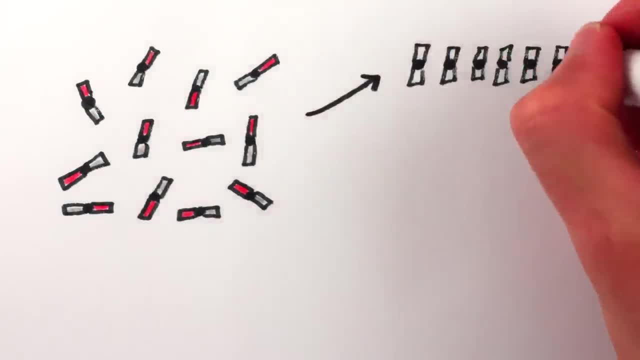 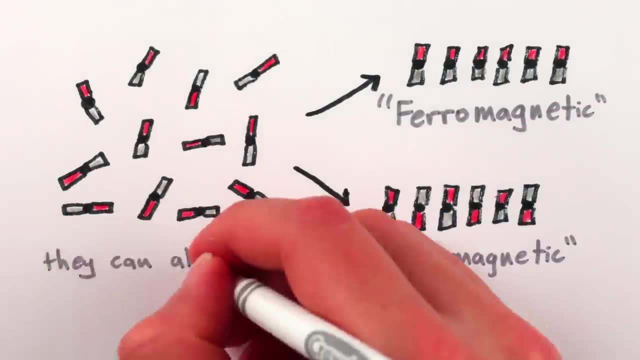 they generally have two options. One is for all the atoms to align their magnetic fields with each other, or they can align their magnetic fields in an alternating fashion so they all cancel out. The atoms will do whichever one requires less energy. That's why chromium, for example, is a very magnetic atom. 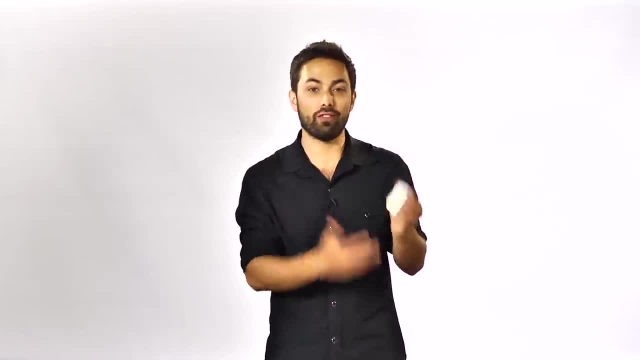 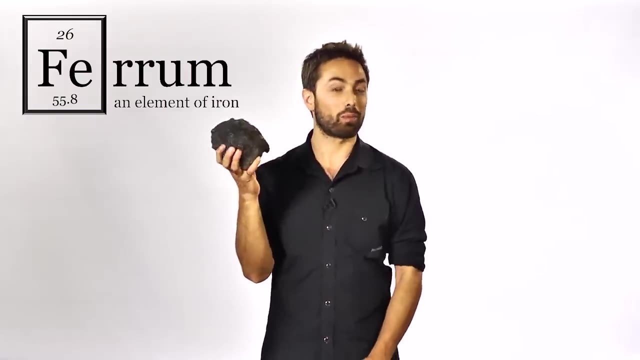 but a very unmagnetic solid, Because it's one of the most anti-ferromagnetic materials that we know. Iron, on the other hand, is the namesake of ferromagnetism, so it is unsurprisingly ferromagnetic, Or, in usual parlance, magnetic. 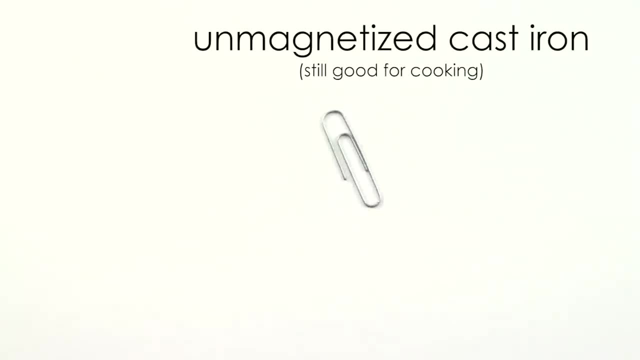 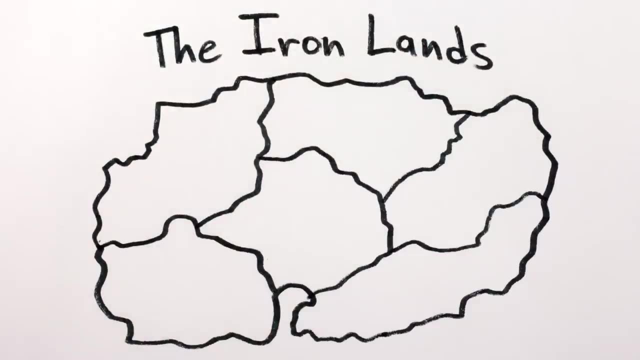 Sometimes The last and final level of magnetism is that of domains. Essentially, even in a magnetic material where the magnetic fields of atoms line up together, it's possible that one chunk of the material will have all its atoms lined up, pointing one way. 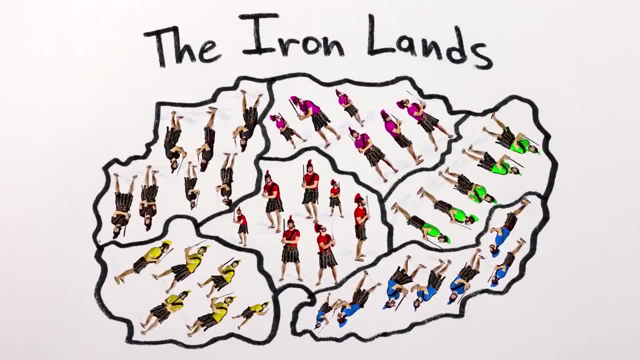 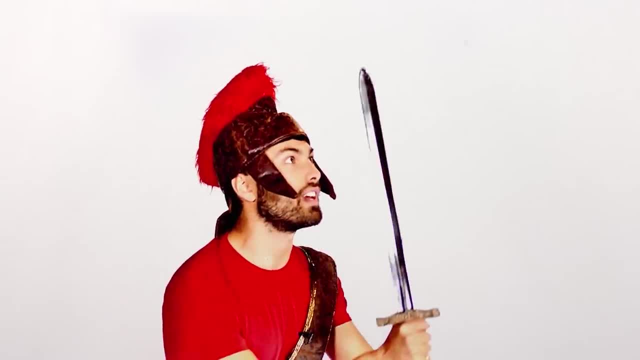 and another chunk will have all its atoms pointing another way, and so on. If all of these domains are of a similar size, then none may be strong enough to force the others to align with it, In which case a piece of iron, for example, may have no magnetic field at all. 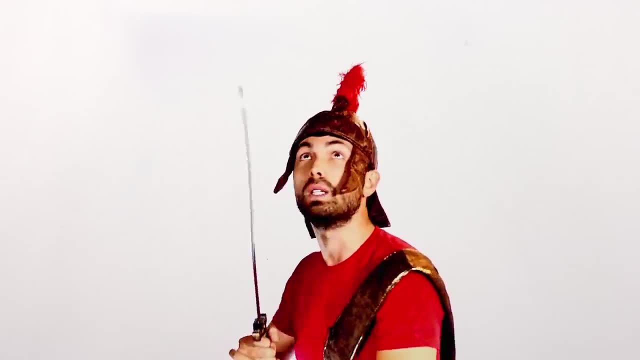 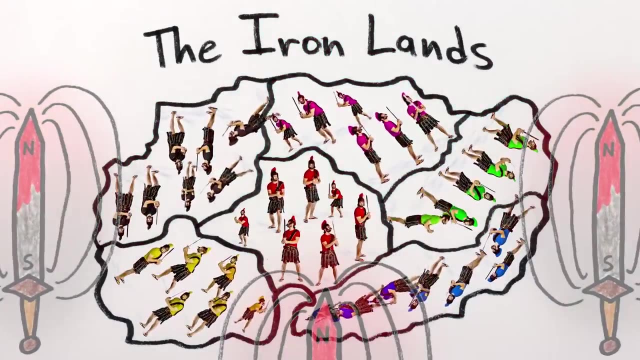 because of all the warring magnetic kingdoms within it. However, if you apply a strong enough magnetic field from outside the material, you can help one domain expand its control over its neighbors, and so on, until all of the domains have been unified into one kingdom. 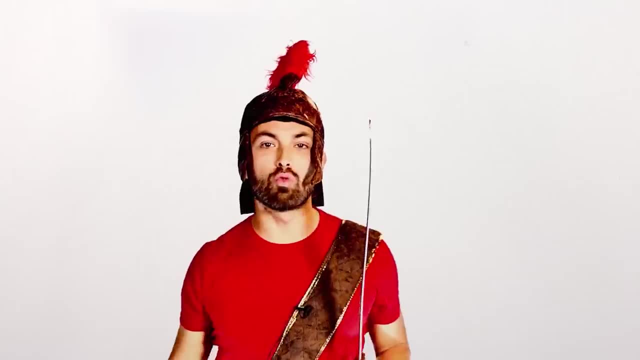 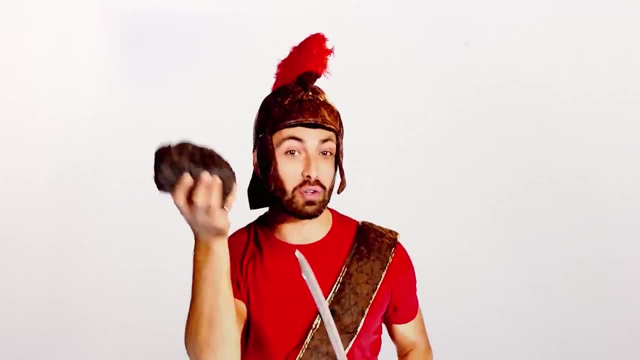 all pointing in the same direction. And now, finally, you can rule with an iron fist. I mean magnet. It's magnetic because it's ferromagnetic and all of the domains are aligned Exactly. What's remarkable is that magnetism is a form of magnetism. 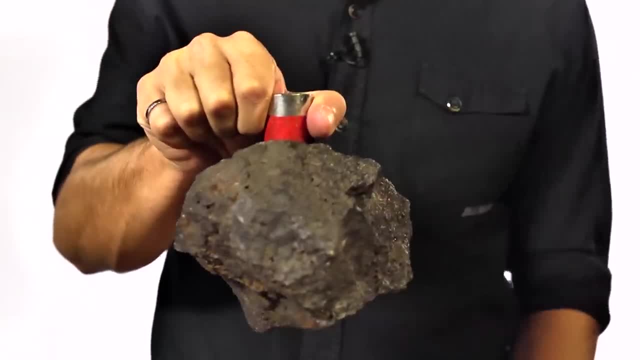 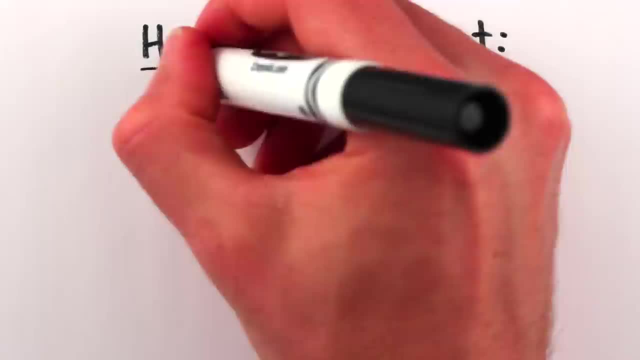 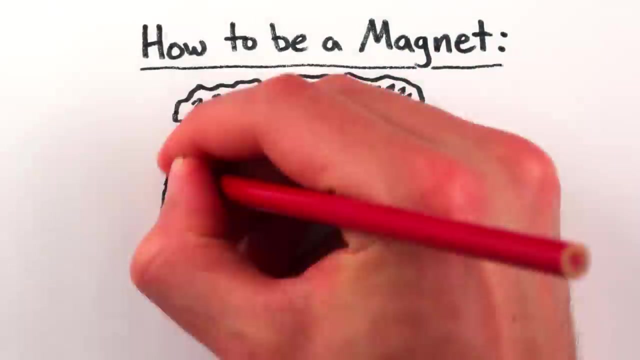 with a fundamentally quantum property amplified to the size of everyday objects. Every permanent magnet is a reminder that quantum mechanics underlies our universe. In order for an everyday object to be magnetic, though, it has to have a unified kingdom of magnetic domains, each made up of bajillions of magnetic atoms, which also need to be aligned with each other. 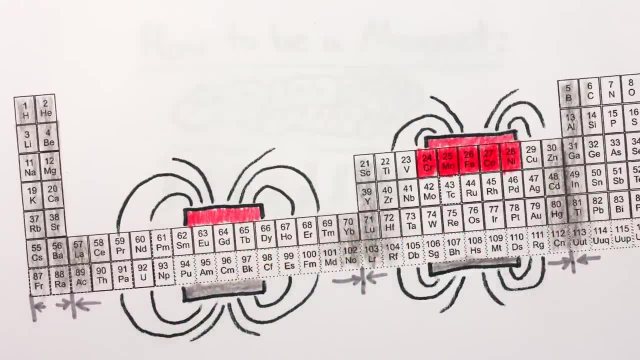 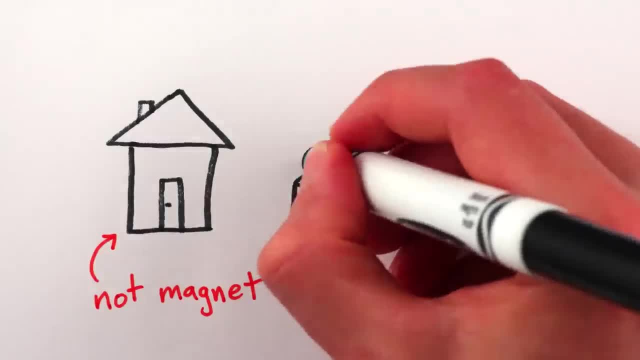 each of which can only be magnetic in the first place if it has an approximately half-filled outer shell of electrons, so their intrinsic magnetic fields can align and not cancel each other out. Not surprisingly, these criteria are pretty difficult to fulfill, which is why there are only a limited number of suitable materials.